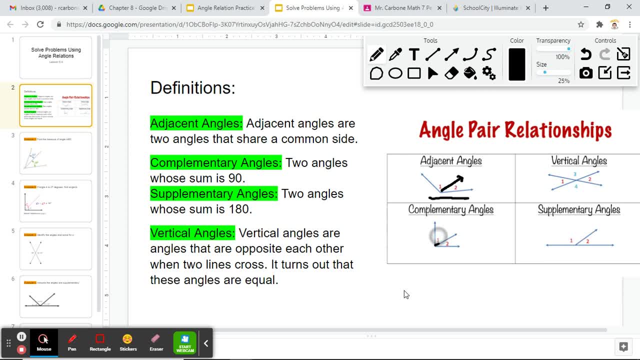 angles are also adjacent angles and where they share the same side. However, now we know that their sum is 90 degrees. So, basically, what do we know? These are, excuse me, these are adjacent angles. If we were bisecting, if we were separating out a 90 degree, 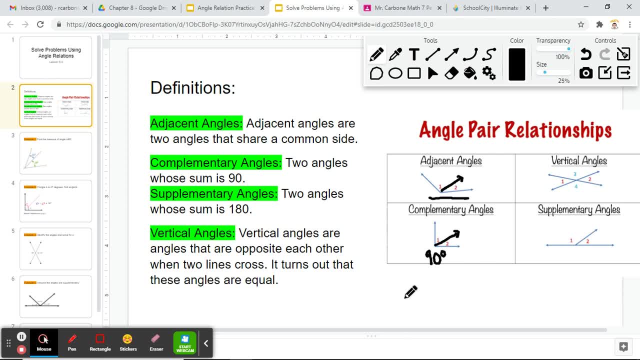 or a right angle. Supplementary angles are also adjacent angles, except now supplementary angles sum is 180 degrees. So if we look at this one here, our large line on the bottom, which is equal to 180 degrees, has been separated out into two other smaller angles: angle one and angle two. 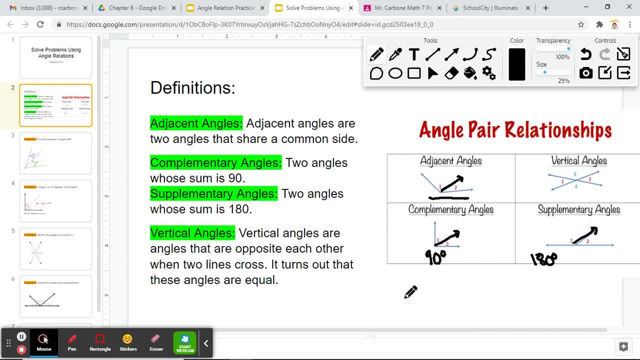 Now the last one we have are vertical angles, And vertical angles are lines that are opposite each other. when two lines intersect, Like we have here, And we know that the angles opposite each other are equal. So, for example, this red one is equal to this red one here. 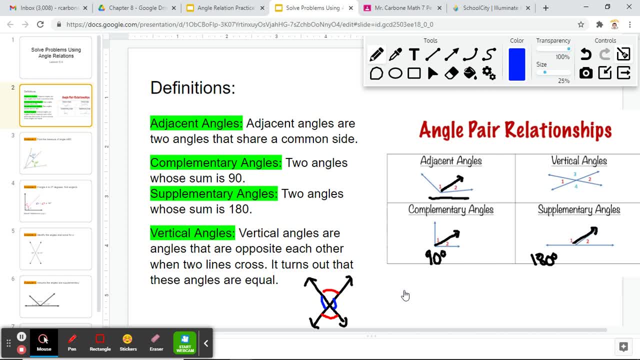 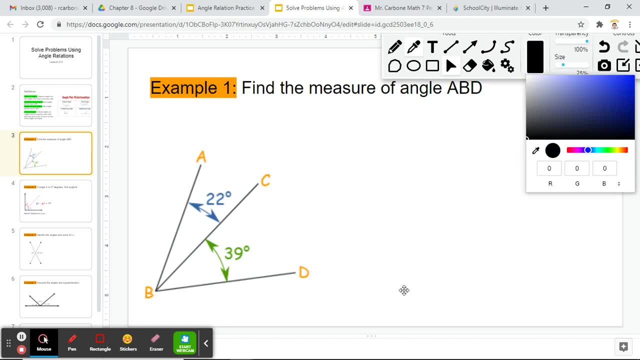 And this blue one is equal to the blue one here. All right, so let's get into our first example for today. We want to find the measure of angle A, B, D. So basically, we want to find the measure of this large angle out here. 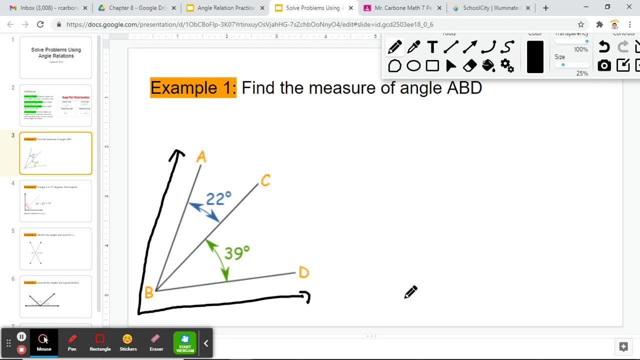 So this large angle is made up of two smaller angles inside, And since they are sharing this common side right here, that means we know these are adjacent angles. So how do we find the measure of angle A, B, D? Well, it's going to be the measure of angle A, B, C, the blue one plus the measure of angle. 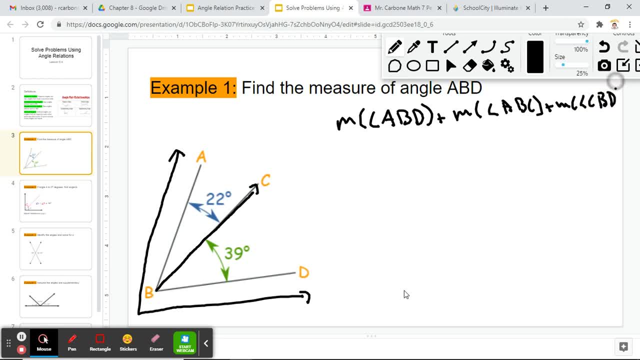 C, B, D, the green one, And that'll be the measure of angle A, B, D. Sorry, they should be equal here. Now that's a little bit confusing way to write it right. So this is basically equal to 22 degrees. 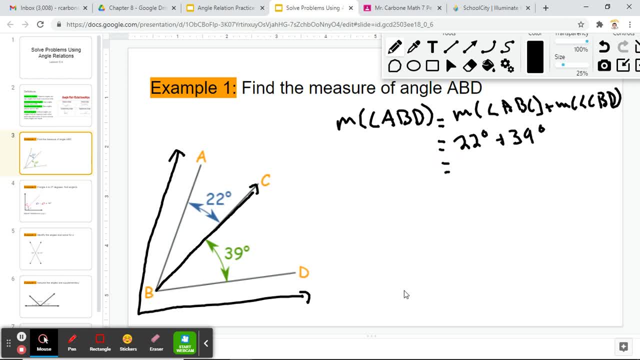 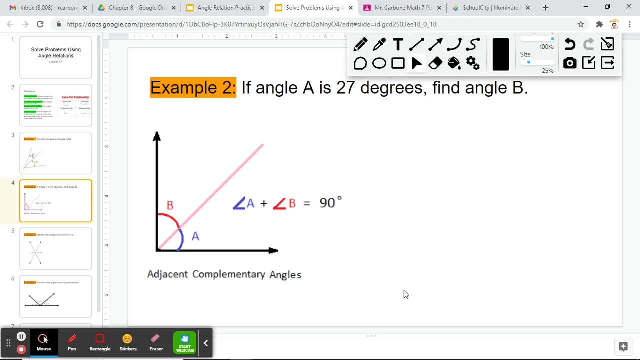 plus 39 degrees, And if we add those together we would of course get 61 degrees. So that means that the measure of angle A, B, D is equal to 61 degrees. All right, another example here. So if angle A is 27 degrees, find angle B. 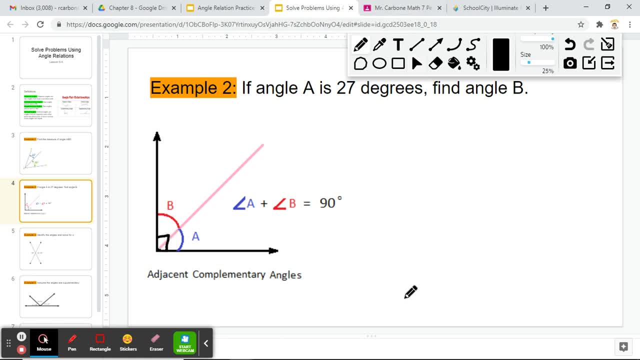 Looking at this figure here, it appears to be a right triangle, So we would assume that this is a right triangle. and then right point triangle looks like a right triangle, so we would assume that this is a right triangle. And since it's made up of two angles, we will call these complementary angles. 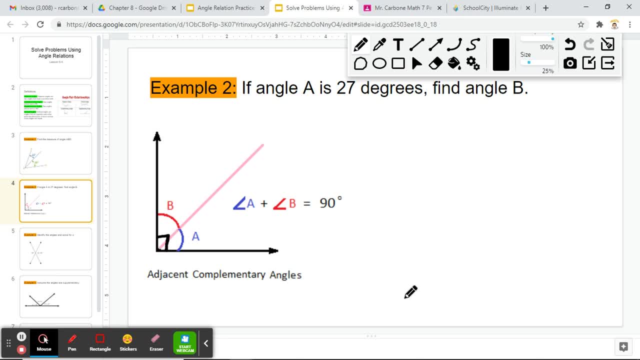 Now this figure tells us that angle A plus angle B is equal to 90 degrees, basically the definition of complementary right. But we could also write that angle B is equal to 90 minus angle A right. You take away whatever angle A is from 90, and that will give you the remainder, and whatever's left will be angle B. 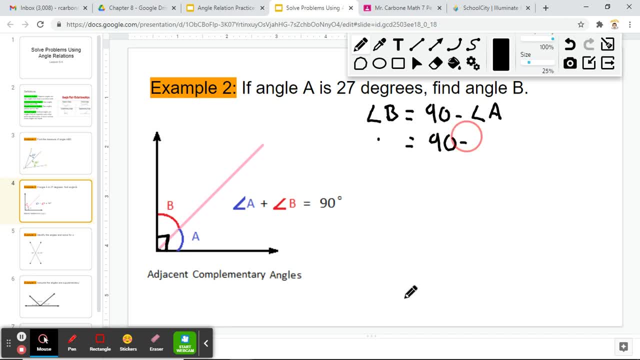 So this is 90 minus. here angle A is 27 degrees. it tells us that right here at the top. So 90 minus 27 would be equal to 63 degrees. so that means angle B is equal to 63 degrees. 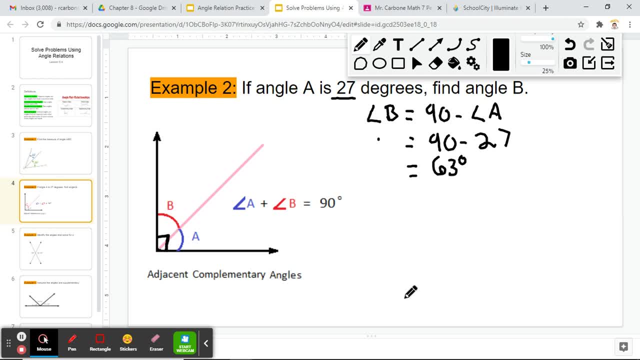 And how do we solve this one? Well, it's because they are complementary angles, so we knew that their total sum, or the sum of both those smaller angles, would be equal to 90.. Alrighty, a couple more examples for us here. 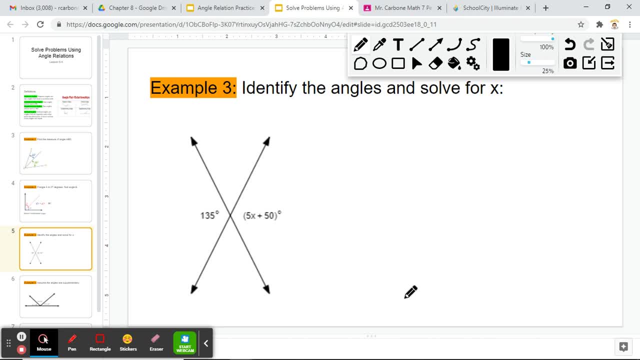 We've got this third one. Well, we have two lines that are intersecting here. So since there's two lines intersecting, that means the opposite angles are equal because they are vertical angles. So these blue ones here would be equal and the red ones all the way out here would also be equal. 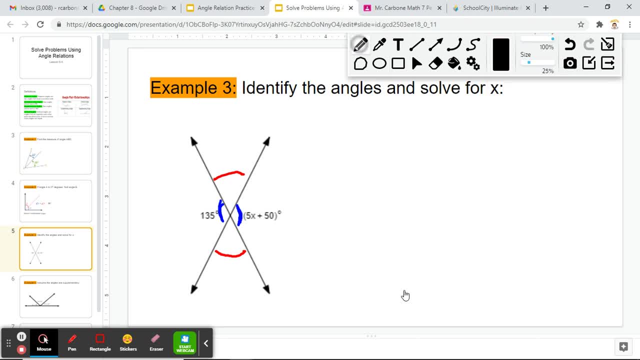 But we don't really care about the red ones right now. it didn't tell us anything about them, so let's just work with these two blue ones. here We can see that 5x plus 50 is equal to 100. So we're going to divide that by 5, and we're going to get 135, because these are both vertical angles. 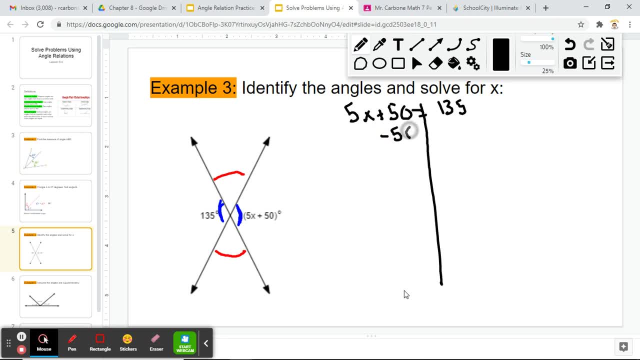 Now to solve this. this is just a two-step equation here, So we'll start off by doing the opposite of adding 50, which is subtracting 50, and we'll do that to both sides. So 50 minus 50 is obviously 0, and 135 minus 50 would be 85.. 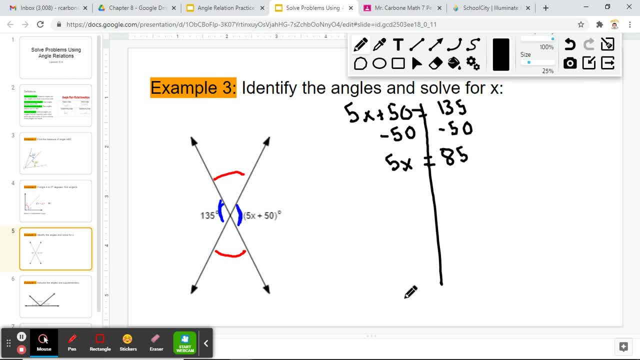 So we get: 5x is equal to 85. Now, since we're multiplying by 5, here we need to do the opposite of multiplying, which is dividing, so we'll divide by 5.. So 5 divided by 5 is obviously 1, so on the left, we get x. 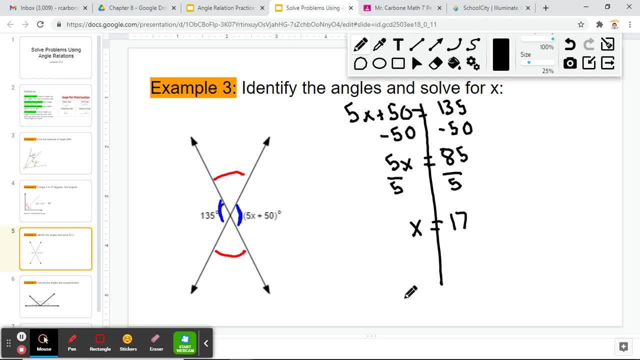 And on the right, 85 divided by 5 is 17,, so we get: x is equal to 17.. Now if I wanted to plug this 17 back in here to double-check my work and make sure I got it correct. 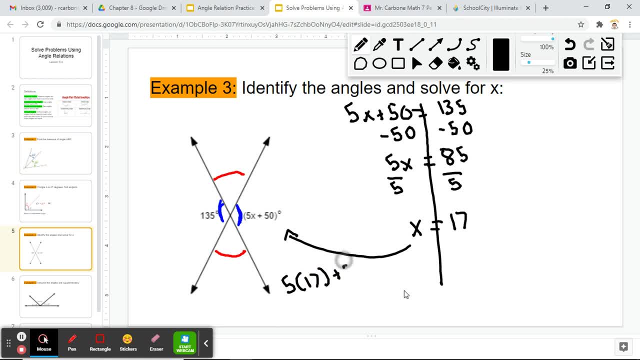 we could do 5 times 17 plus 50,, which is equal to 85 plus 50,, which is of course equal to 135.. So we can see that these two angles here are indeed equal. All right, we've got one more example left for us here. 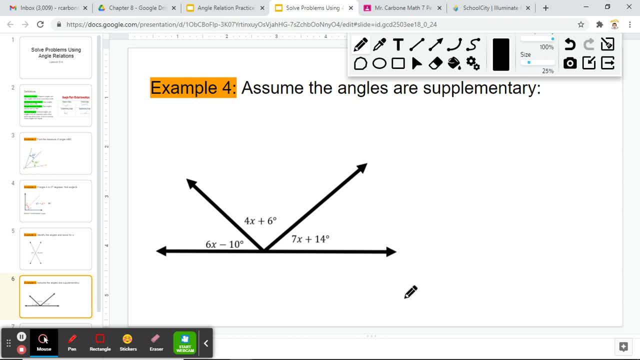 We want to assume that these angles are supplementary. Well, since they're supplementary. we want to assume that these angles are supplementary. Well, since they're supplementary, that means they're all going to add up to 180 degrees. So what do we need to do? 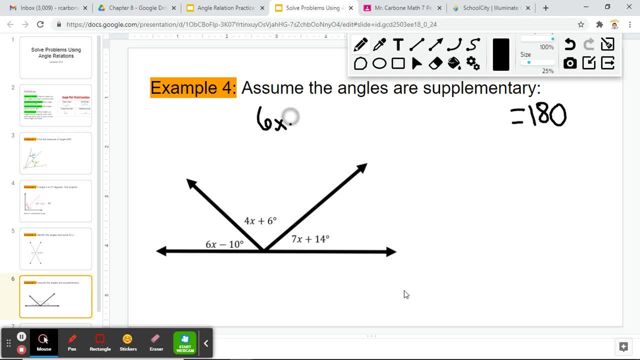 Well, we literally just need to add these three angles together, So we have a 6x minus 10 plus 4x plus 6 plus 7x plus 14.. And once we add all of those angles together, they'll be equal to 180. 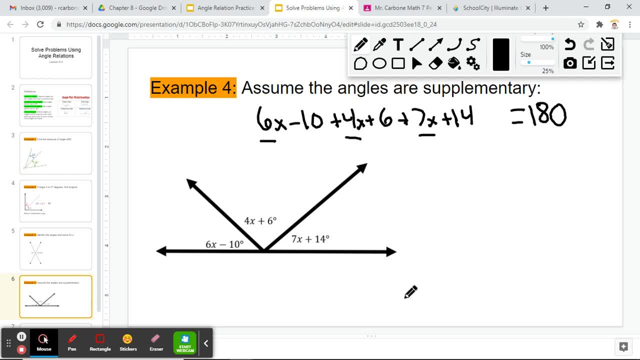 So, looking at these here, we have a bunch of different terms with the same variables, So these are like terms. What do we do when we see like terms? We combine them. So to combine like terms we just need to add the coefficients or add the numbers in front. 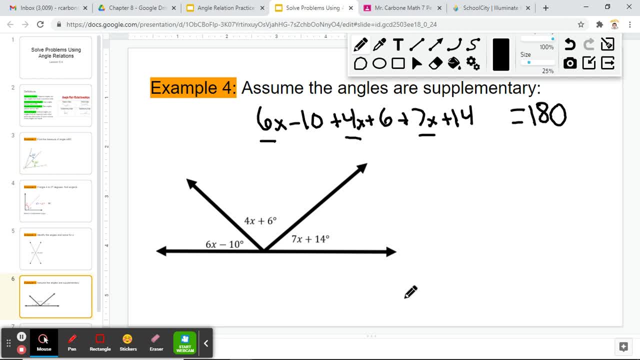 So I have a 6x plus 4x plus 7x. That's the same as 6 plus 4 plus 7, which would be equal to 17x. Next, I have a negative 10 and a positive 6.. 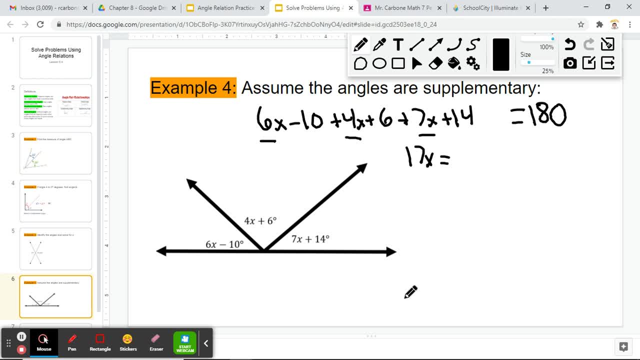 So negative 10 plus 6 would be negative 4. And then I have a negative 4 plus a positive 14.. Negative 4 plus positive 14 would give me a positive 4. And that would be equal to 180.. 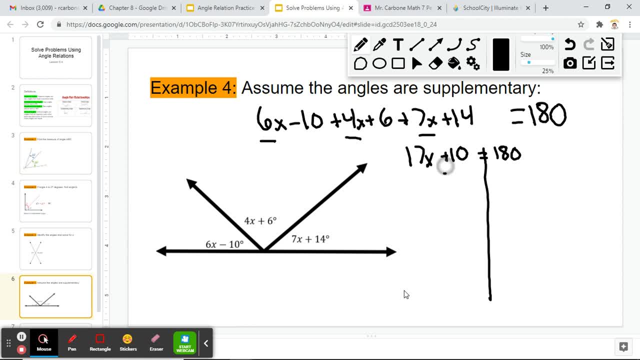 So again, just a two-step equation for us to solve here. The opposite of adding 10 is subtracting 10.. So we'll do that. from both sides We get a 17x is equal to 180. minus 10 would be 170.. 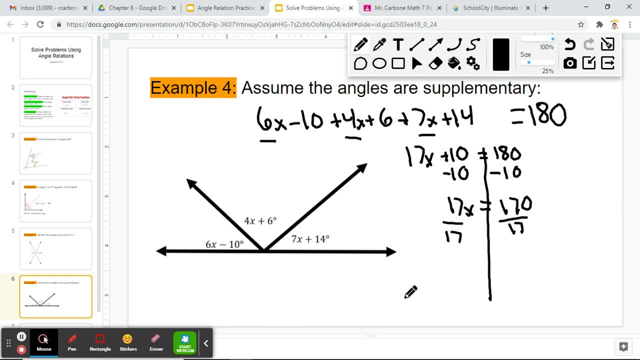 And then, when we do the opposite of multiplying by 17,, which is dividing by 17,, we'll divide both sides by 17 and get x is equal to 10.. And that is our answer to our problem here. All righty. 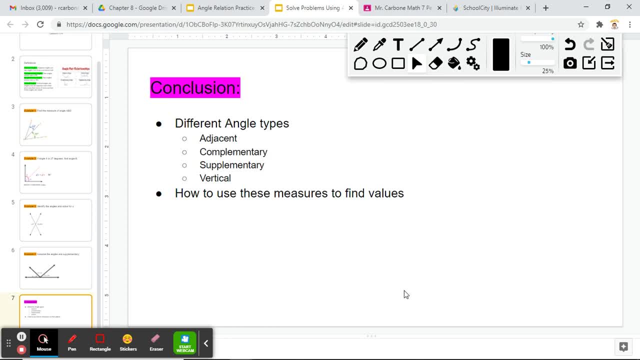 So, for our conclusion today, what did we learn? Well, we went over some different angle types. right, We talked about our adjacent angles, And adjacent angles are just two angles that share the same side: Complementary and supplementary are both adjacent angles. 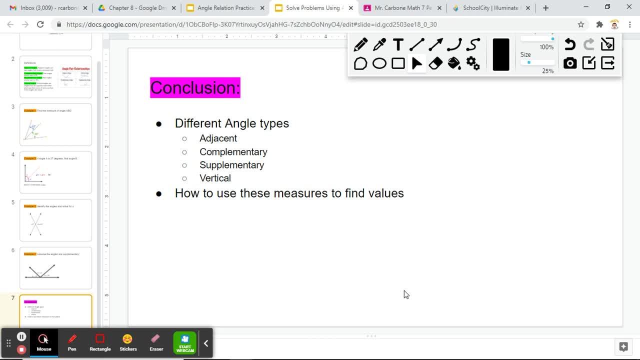 However, complementary specifically has to do with 90-degree angles And supplementary has to do with 180-degree angles. And lastly, we talked about vertical angles, And that says whenever two lines intersect, the angles opposite each other are equal. Lastly, we used those angle measurements. 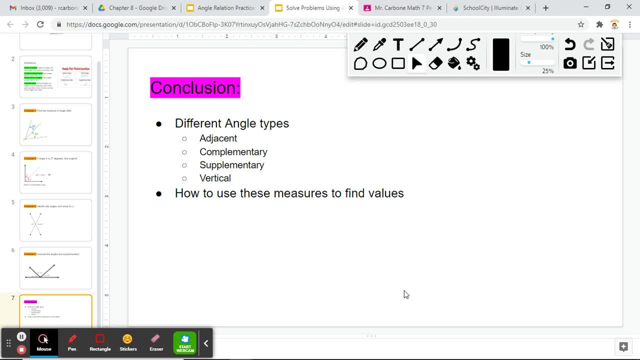 And those angle relations in order to find values, whether it be through algebra, through just setting it up or simply just doing some simple addition. All righty, everybody, That was our notes for today. Make sure you're getting these down and asking those video questions –.